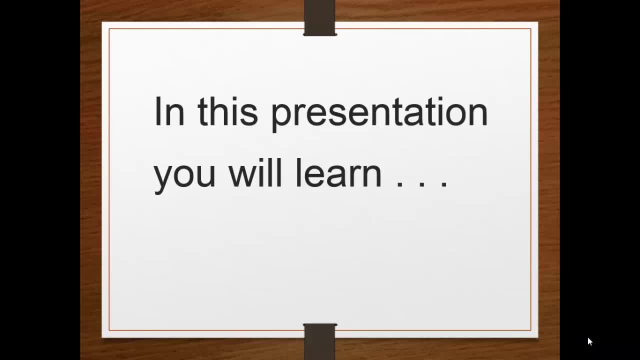 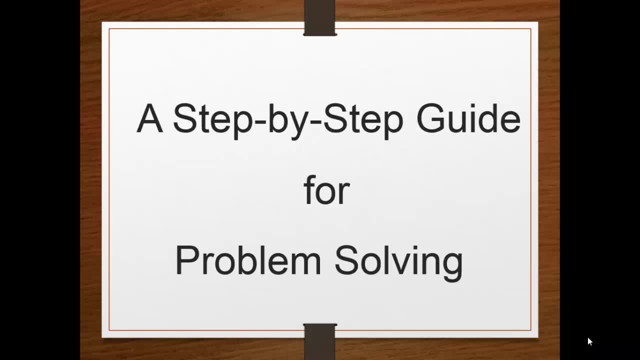 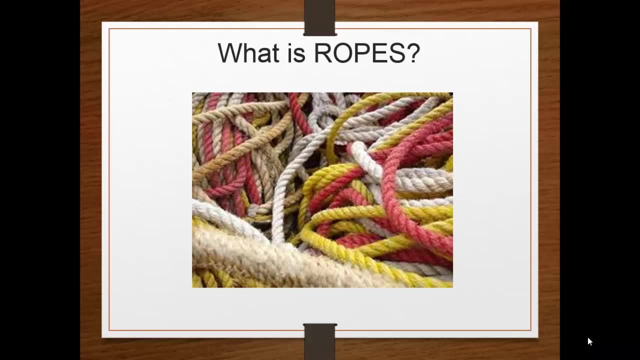 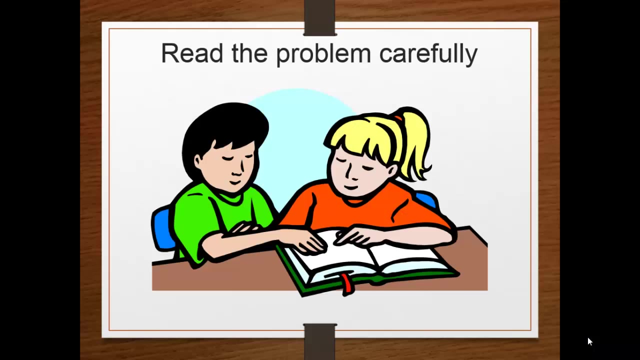 ROPES is an acronym for the five problem-solving steps you can use to solve a word problem. The first letter in each step stands for one of the letters in the word ropes. Let's take a look at the steps. Don't assume you know what the problem is asking by taking a quick glance. 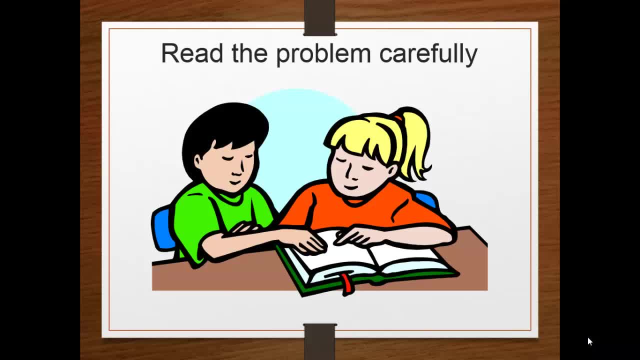 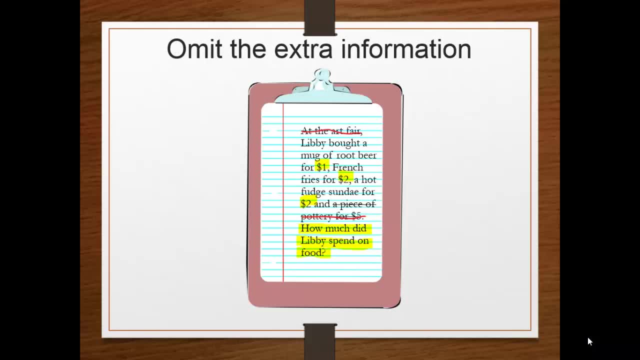 Make sure you read the problem at least two times. Be sure you are reading to the last punctuation mark. Word problems often have information that is unnecessary. This extra information is called a distractor. These distractors are put there purposefully. Don't fall for the problem writer's tricks. 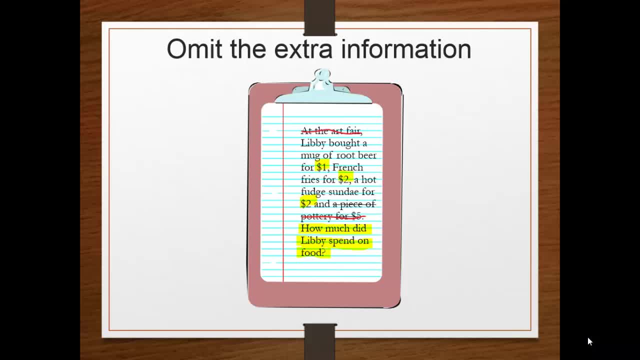 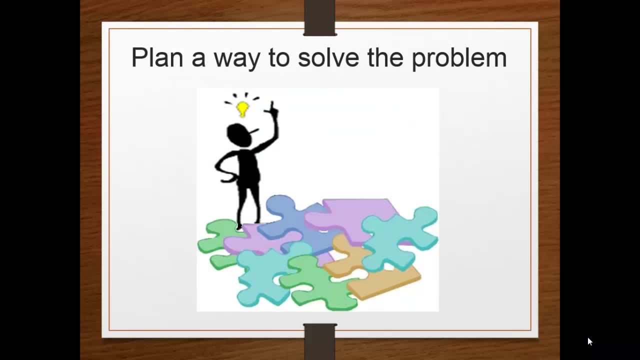 Cross out information that is not important. Highlight, underline or circle the important information so you don't forget it. Before you start working, make sure you understand how the facts in the problems are related to each other. Remember there are many ways to solve a problem. 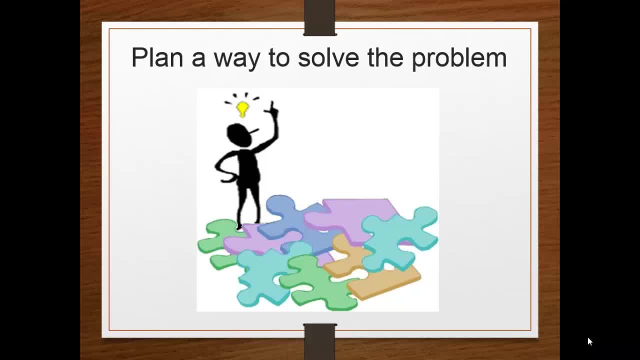 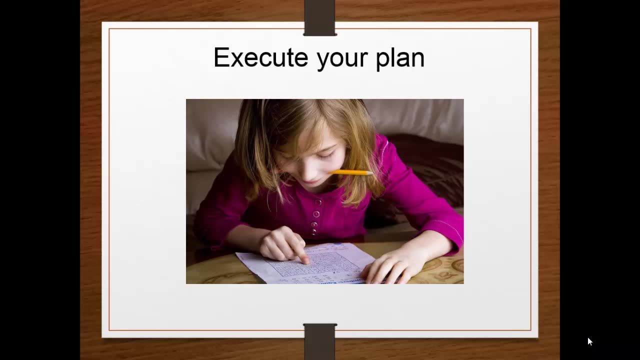 Try one of the problem-solving strategies that you have learned in class. Before you start working out the problem, try to estimate the answer. This will help you know if your plan was successful. Carry out your plan. Don't try to work out the problem in your head. 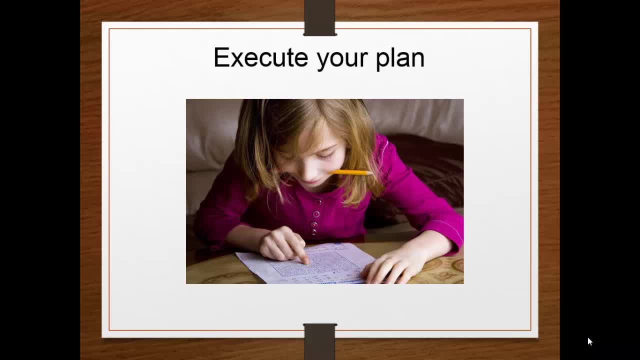 Write down your work. Even if it seems like a lot of extra work, it really will help you avoid making silly mistakes. Plus, you can go back and check your work If you need to revise your plan. having your work written down will help you come up with a new plan. 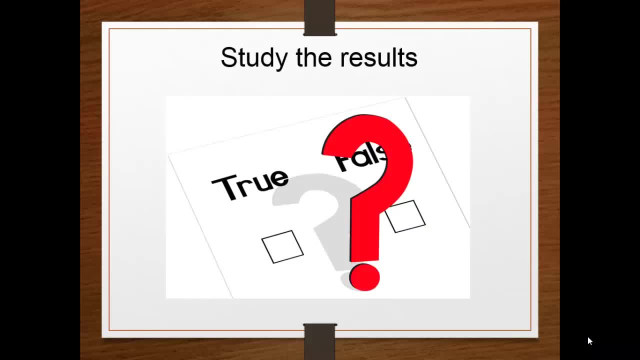 And after you have carried out your plan, look at the answer and ask yourself if the answer seems reasonable. Please don't skip this step. Are you sure the answer you have answers the original question? Does your answer match your estimate? If you can't say yes to these questions, 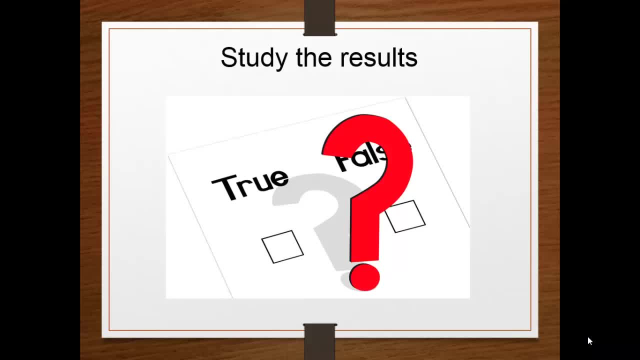 you need to go back to the beginning of the problem-solving process. Good luck.